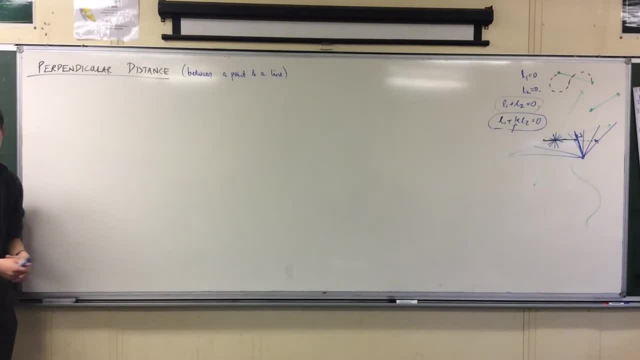 and the shortest. And the shortest distance is the perpendicular distance, Just like if you're crossing a road, the fastest way to get across is to cross perpendicular to the direction of the road, rather than kind of go at an angle right. So therefore, that's what perpendicular distance is referring to. 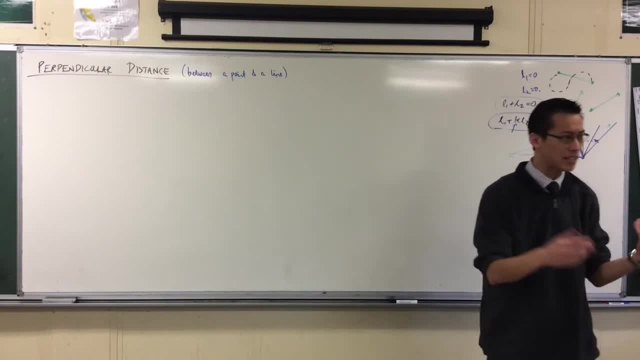 Now I'm going to do something a bit unusual, which is I'm just going to give you what the formula is right off the bat, okay, And then we're going to prove it after that. I usually like to do it the other way around. 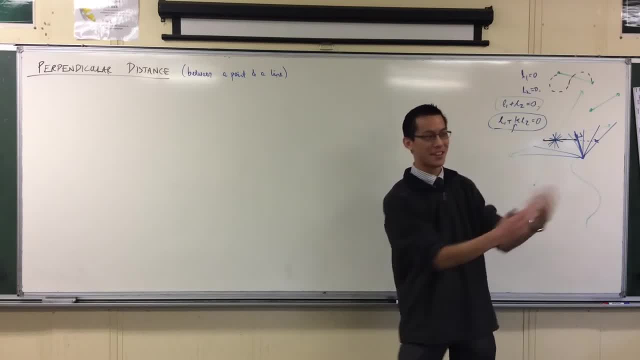 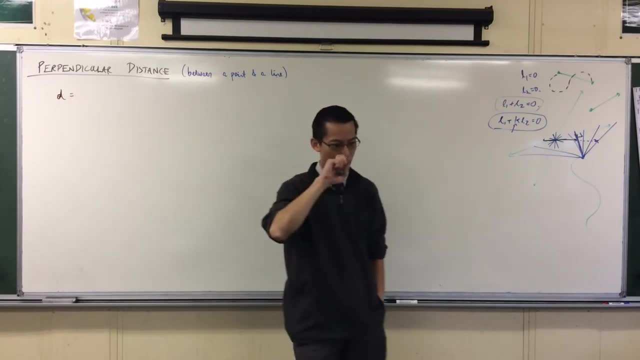 because it's kind of like you know logic. Where does the formula come from? It comes from the proof, Because the formula, as you'll see- and some of you are familiar with it- looks quite awkward. I'm just going to give it to you. 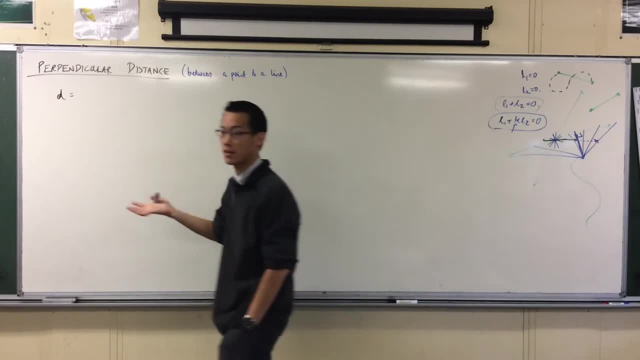 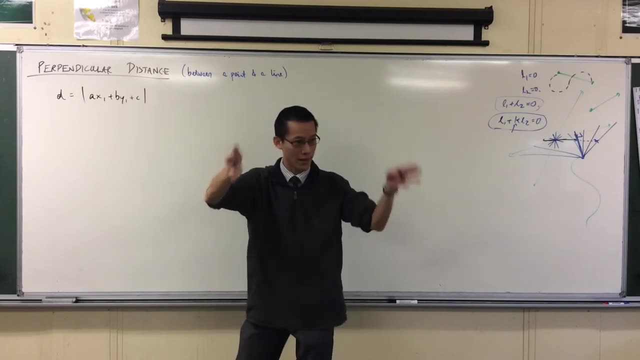 so that when we prove it you'll be like: oh okay, I can see the pieces starting to form. So here's the formula. It's the absolute value of ax1 plus by1 plus c, absolute value all over the square root of a squared plus b squared. 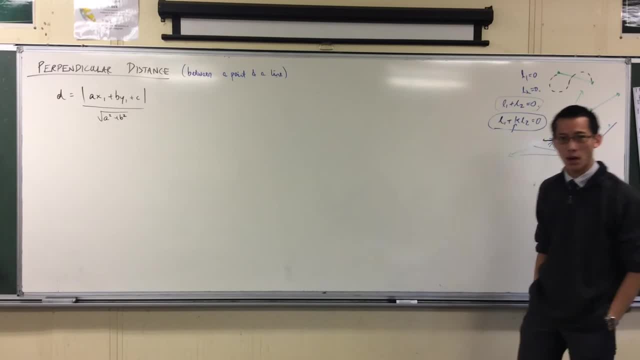 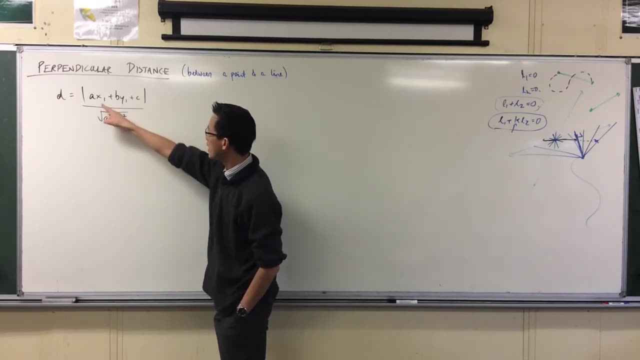 So there's a couple of things to note. You have a look at it. What are the pieces that go into this? The first easy piece to identify is: you've got x1 and y1, which clearly are talking about this point right. 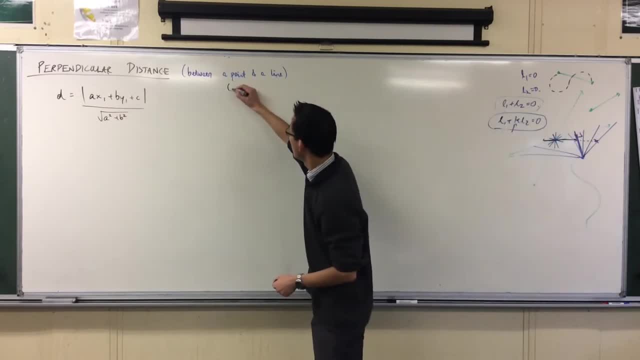 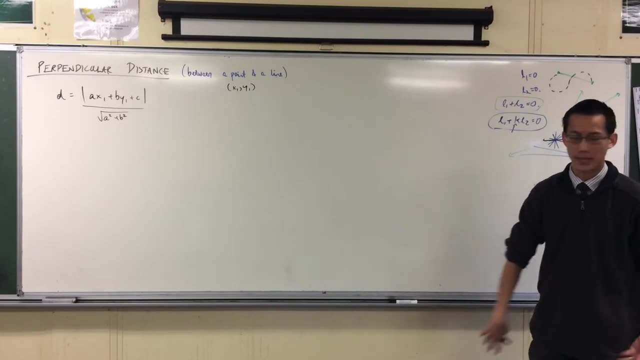 So when there's like some point and some line, the point is x1,, y1,- right, Not to be confused with x and y, which are variables, right? So this is some actual values. When you look, what are the rest of the pieces? 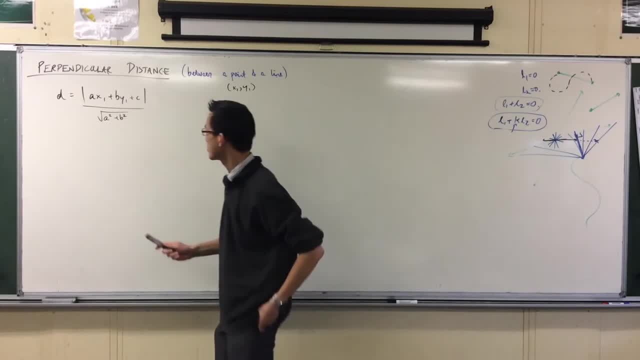 Don't get overwhelmed by how much stuff there is. Yeah, The square root of a squared plus b squared is because it's perpendicular and there's a 90 degree angle. Okay, Okay, good, It's Pythagoras. Good, good, good. 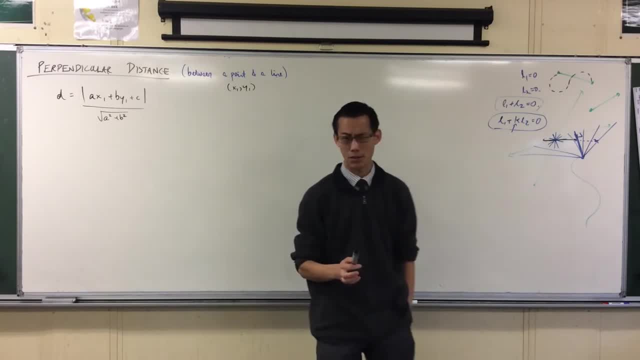 When you look at this like that's always going to make you raise an eyebrow and say: what's going on with that? Clearly, Pythagoras is involved, and the reason Pythagoras is involved is because there are things that are at right angles. 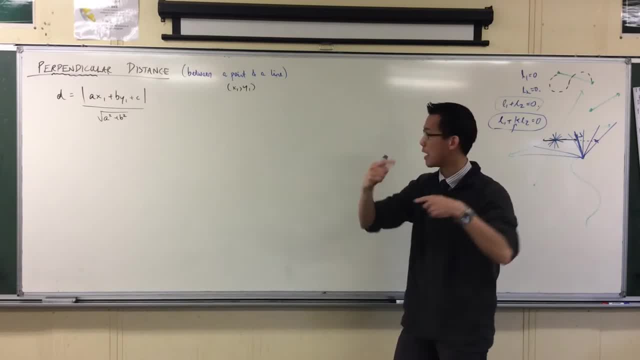 Okay, so we'll get to that. As for the pieces that go into Pythagoras, you've got a, b and c. What do you think the a, b and c stand for? Yeah, The formula for the line. 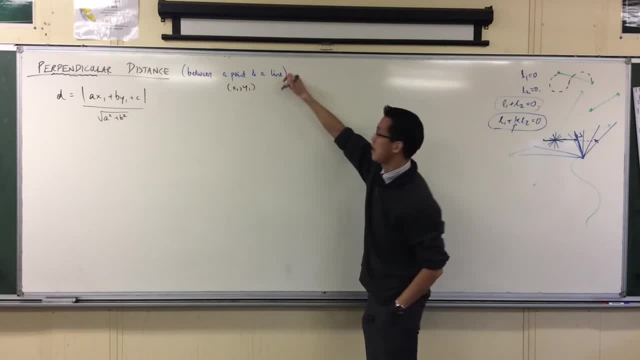 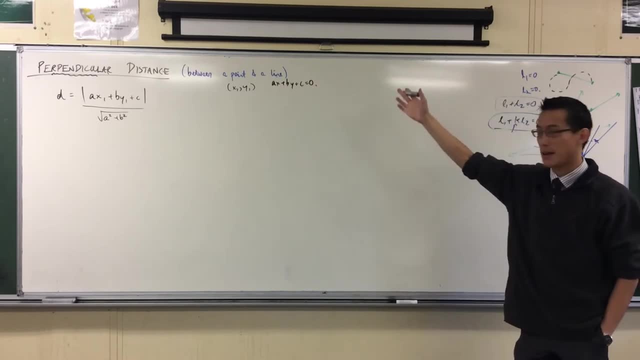 Yeah, good, We've already got the point covered, right. We want the line, and so that line is ax plus by plus c equals 0. General form: okay, So that's the a, b and c. that are these a, b and c. 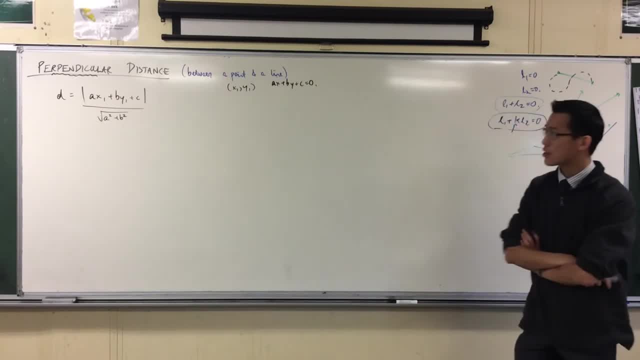 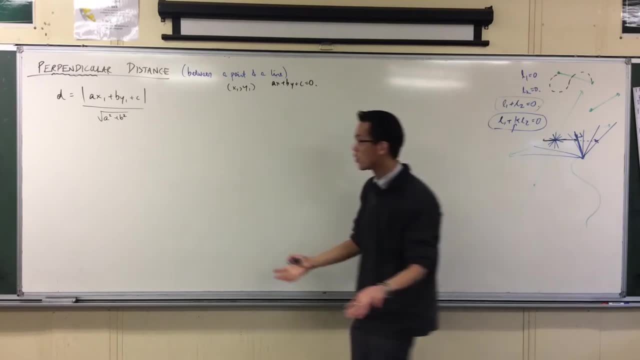 Okay, so there's the formula. One other little thing to notice: there's an absolute value there on the numerator. Why is that? Because it's a distance, right. So I want a positive value, As opposed to that other distance formula that you know, where you just have two points right. 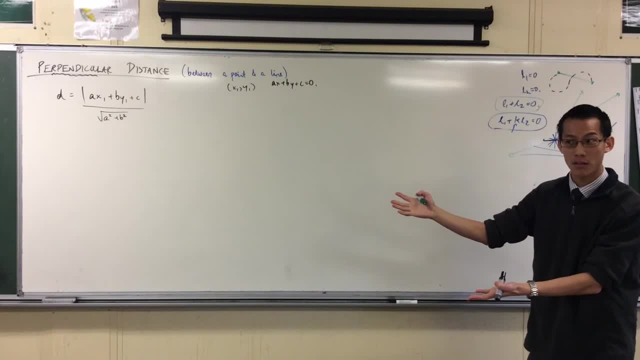 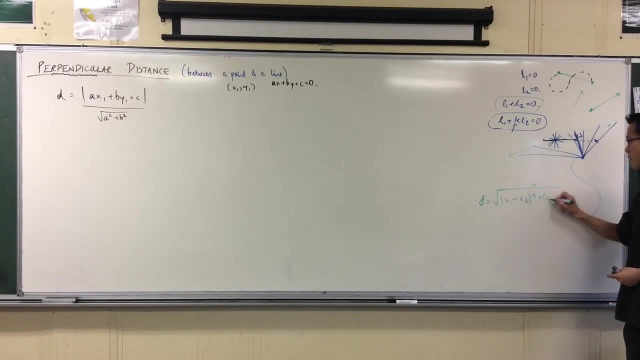 The other distance formula doesn't have an absolute value. sign on it because Because it's just a square root, It's a square root, It's a square root, It's just the square root of this plus this. So by definition it's positive, right. 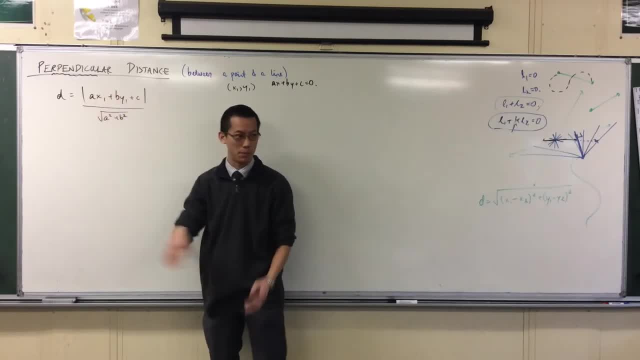 But, as you can see, it doesn't take that much effort to pick out a combination of a's and b's and c's and x's and y's and y's, such that you get a negative on the top and you'd be like 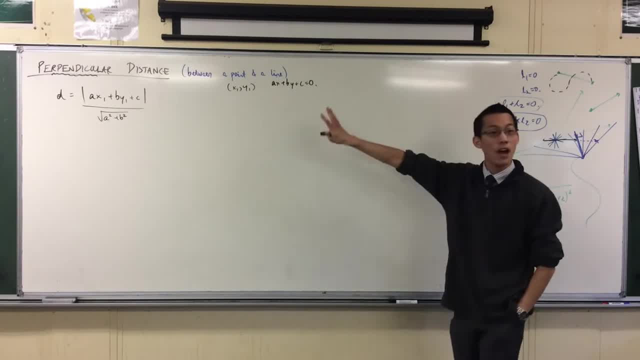 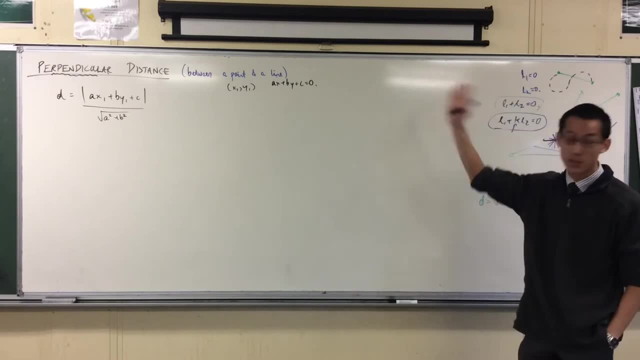 uh-oh, you know I want a distance, okay, So that's where we're going to end up To get there. your textbook has a proof of this result. There's loads of proofs of this result. It's a good proof. 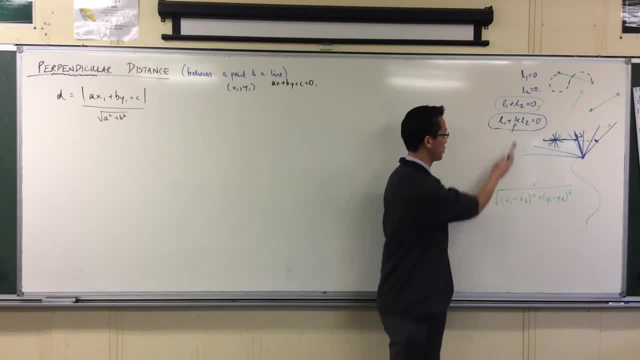 It's very algebraic, It's very algebra-heavy, And I'm very conscious of the fact that you've been doing quite a little bit of algebra already, right? So here's what I'm going to do. instead, I'm going to show you a slightly different proof. 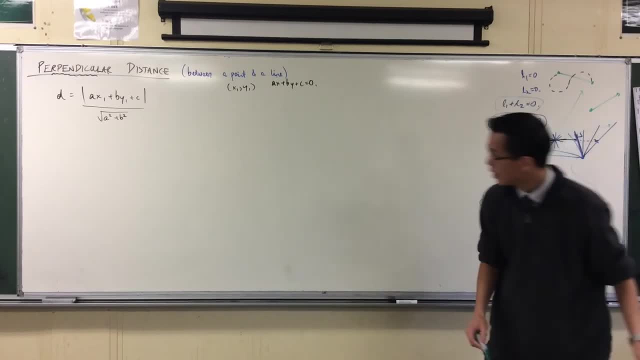 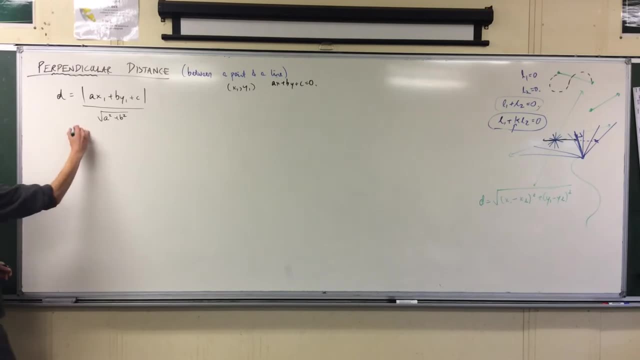 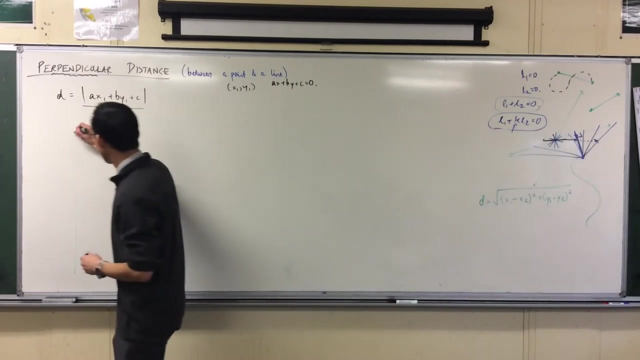 You'll need a set of axes, so draw one up with me, Just for simplicity's sake. let's just do a basically first quadrant diagram. So that's not a good pen to use. We could use more quadrants, but we only need one. 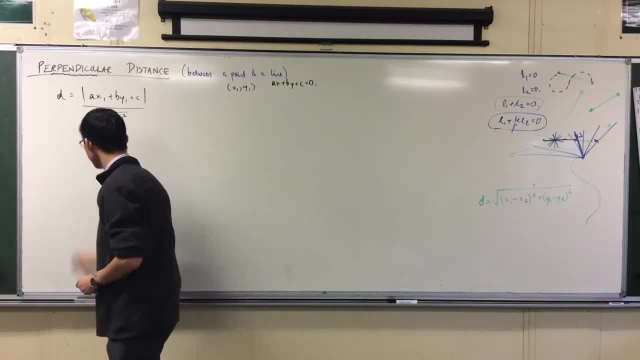 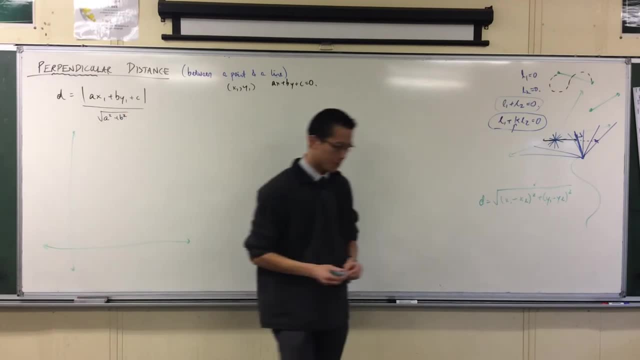 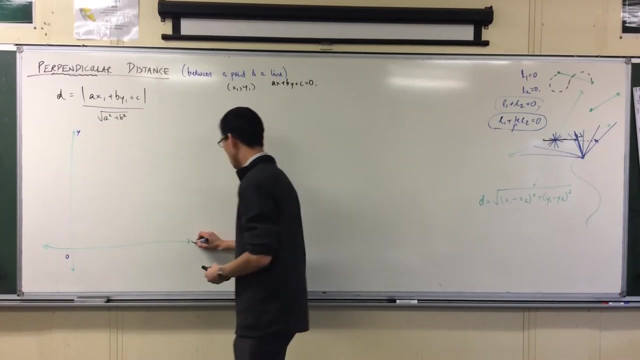 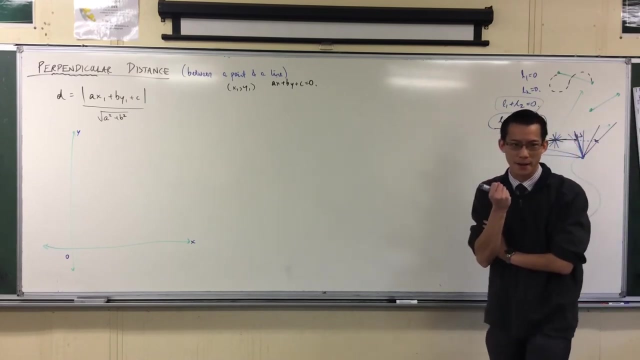 We don't have time to really illustrate what's going on. All right, so here's my first quadrant. roughly speaking, I said that I'm trying to avoid a proof that's super algebra-heavy. Obviously, we're not going to avoid algebra completely, because it is algebra right. 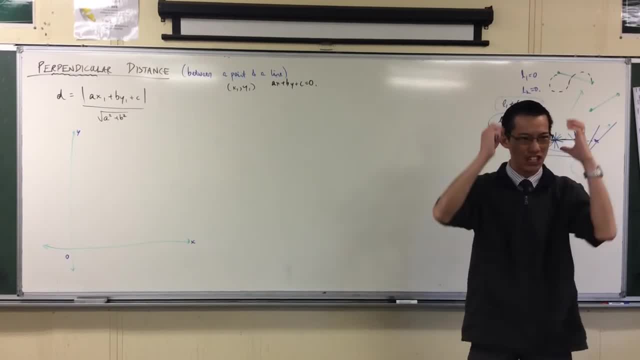 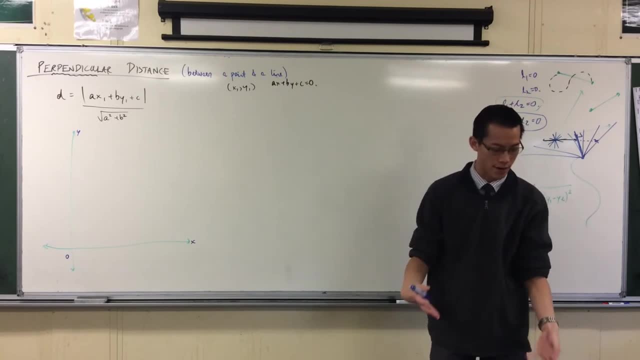 But what I'm going to try and do is try and flex your geometric thinking muscles. okay, This is going to be more visual-heavy and reasoning-heavy than algebra-heavy. In fact, in terms of sheer lines of working, it's about a third the length of the other proof. okay. 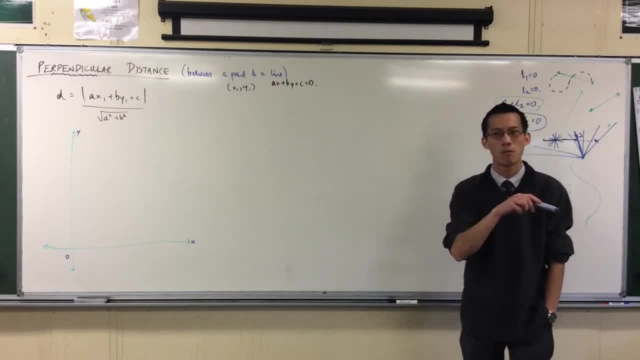 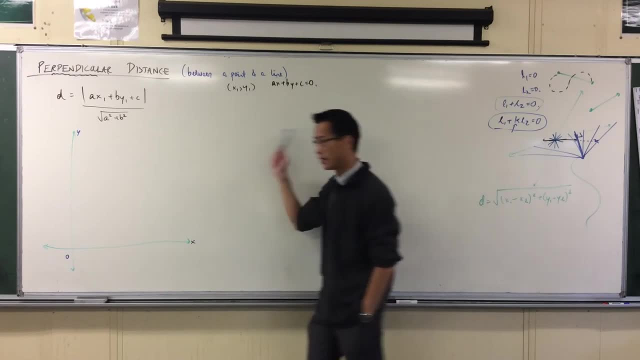 But you have to think a bit harder to see where the pieces come from. So that's the trade-off I've made In our first quadrant. let's draw a particular point and a particular line. Now I have to have It looked into a particular example. 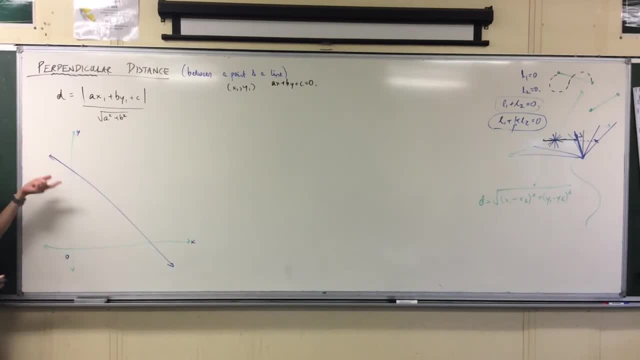 So I'm just going to put a line like that. I'll call that my ax plus by plus c, And I'm going to pick a point. And just because I've got space over here, I'm going to pick the point over here. 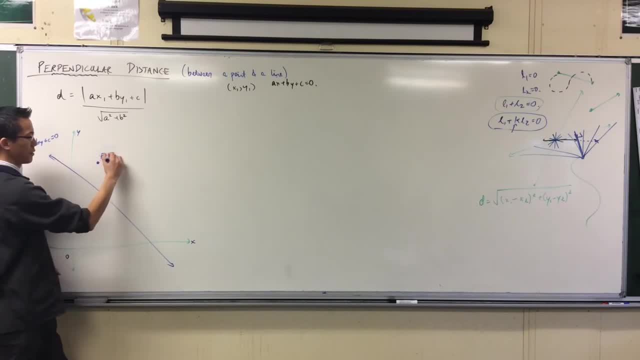 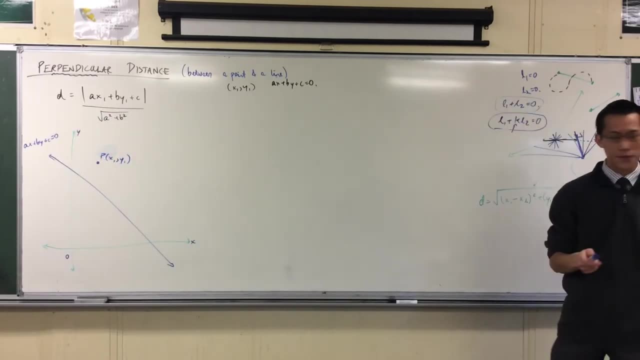 Let's call this. Let's call it p for point, And its coordinates are x1, y1.. All right, so far, so good. So what I'm after is the distance that's shown here, The shortest between this point and this line. 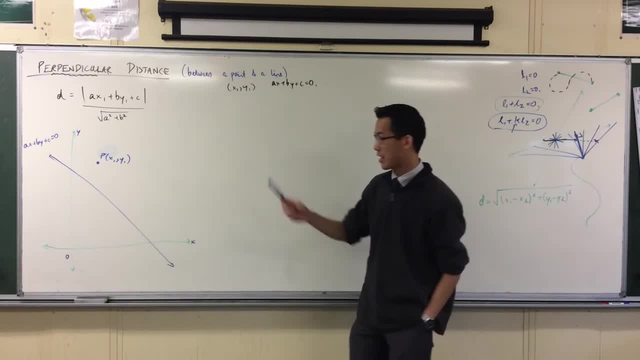 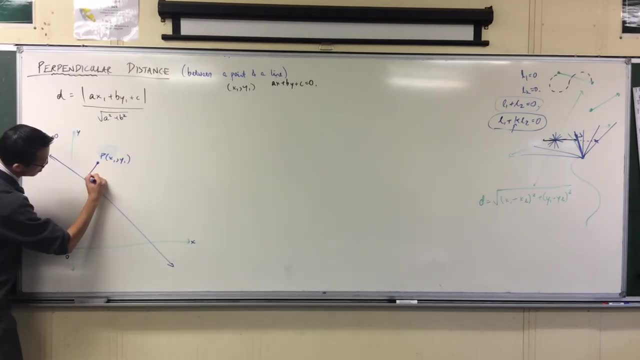 And you can draw it on right. It's the distance, such that you draw an interval so you get a right angle with the line. It's going to look like this And there's our right angle. Okay, that's the actual distance that I'm after. 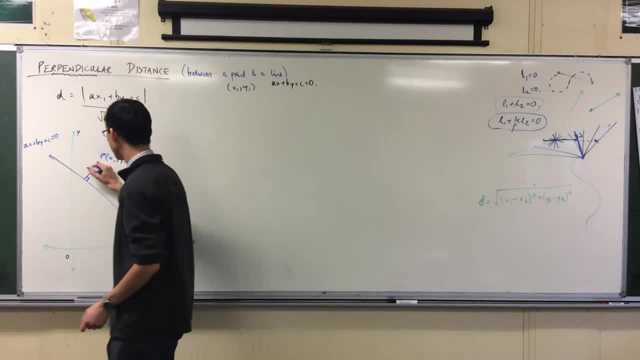 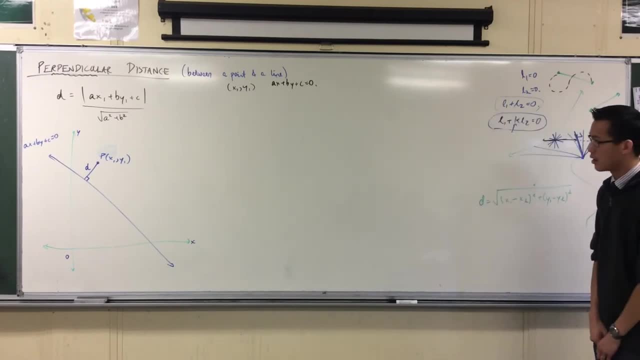 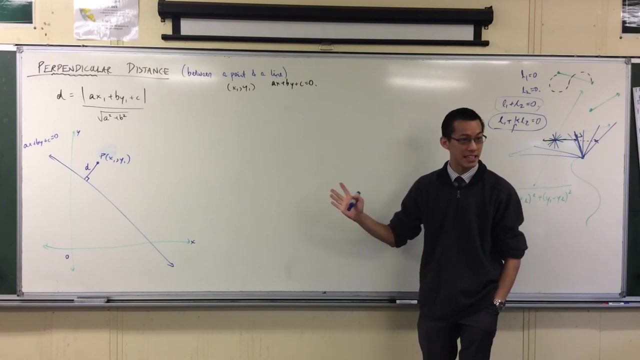 So I'm going to call that distance d Lowercase. All right now. Where are we going to go from here? I need to know a couple of pieces here. I'm going to add some pieces in here which seem a little bit arbitrary. 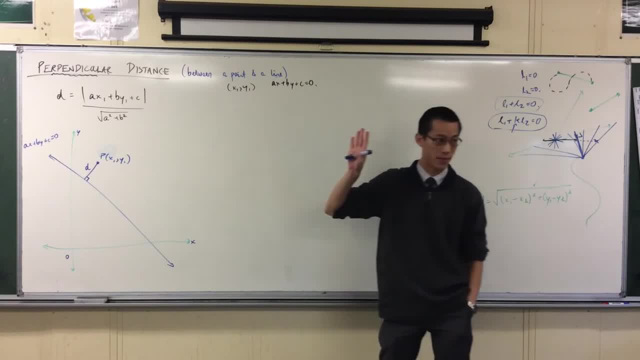 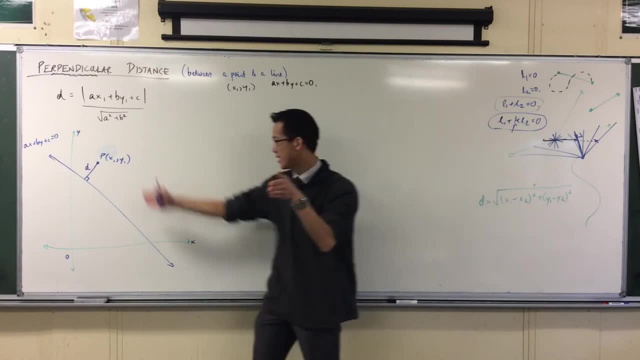 but you'll see the direction I'm going in and how I'm trying to use these geometric features to my advantage. Okay, So from my point p I'm going to drop a vertical line down from p down to my actual line that I'm interested in. 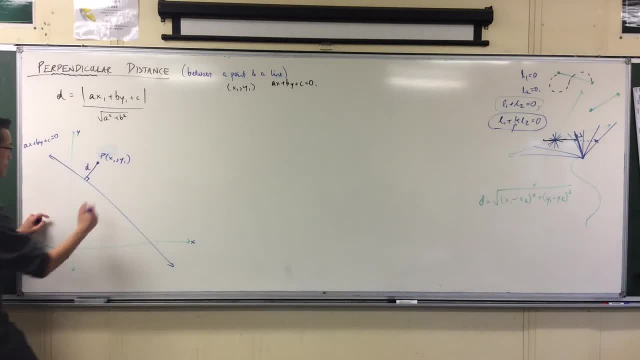 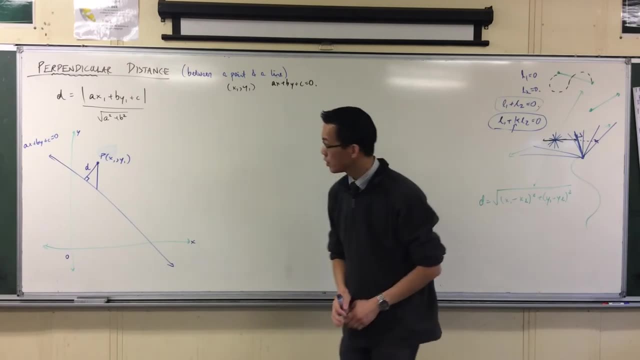 So it's going to be vertical, parallel to the y-axis. So on my diagram it's going to look something like this, Like that, Okay, so what I have formed is a triangle, and I'm going to do some work with this triangle. 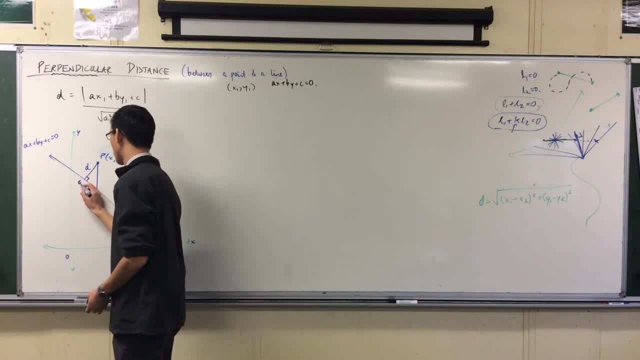 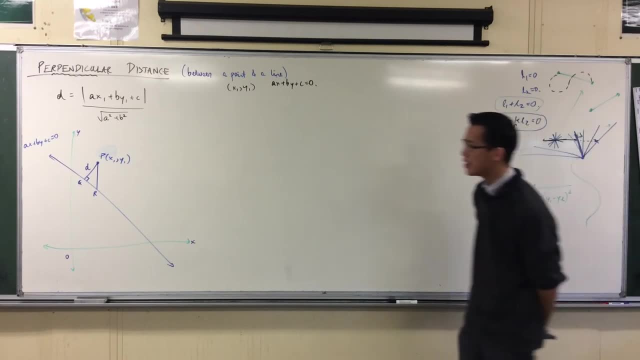 so I want to label it. I want to have some names here that I can talk about, So I'm going to call it triangle p, q, r. All right, Now if this line is vertical, right? just for the sake of clarity.